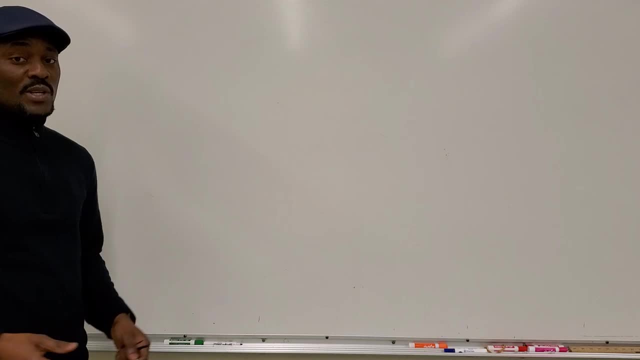 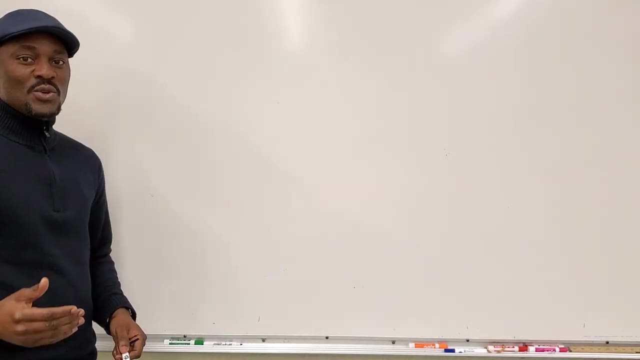 or you have learned or gone through eighth grade in school. you're expected to be able to solve most of the questions that I'm going to show you today. It's just a matter of you trying to be able to solve them. So the very first question that I am going to present- and you're going to get more- 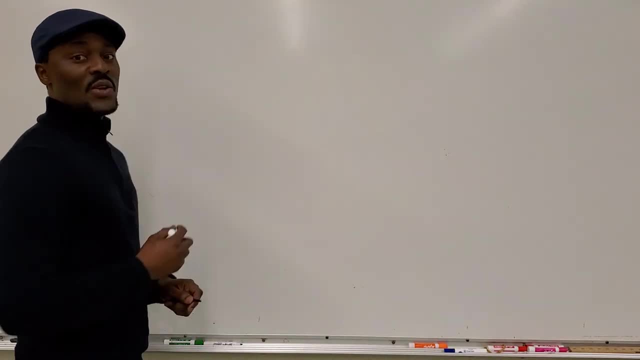 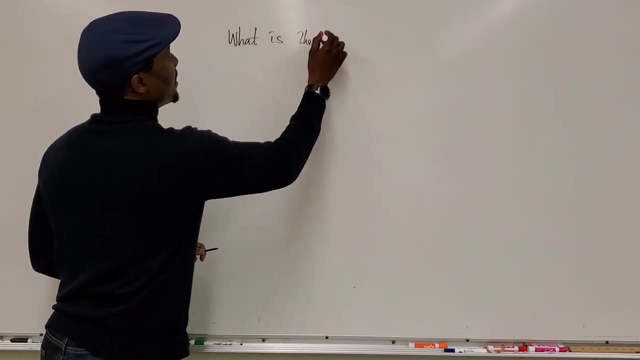 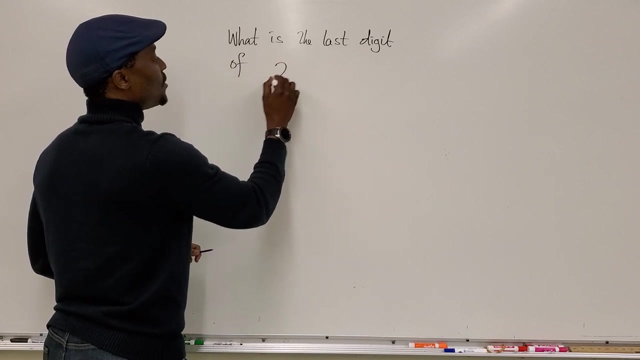 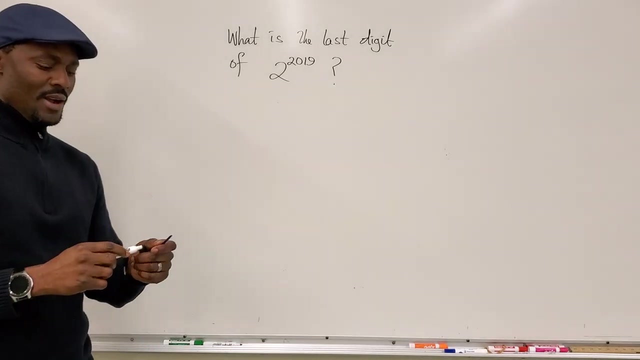 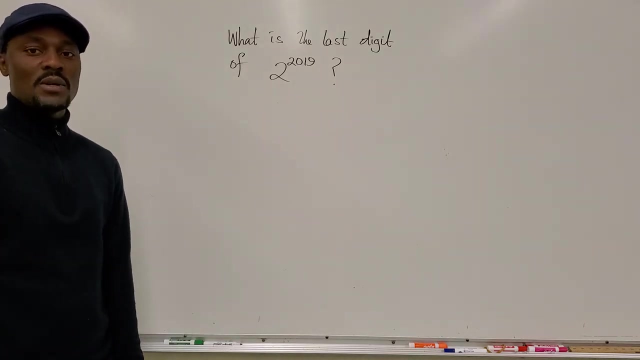 of these kinds of videos over time is a question that looks like this: What is the last digit of 2 to the power of 2019?? So you get a question like this and you go: how do they expect me to know what the last digit would be if 2 is raised to the 2019th power or 2 to the 2019th? Now that 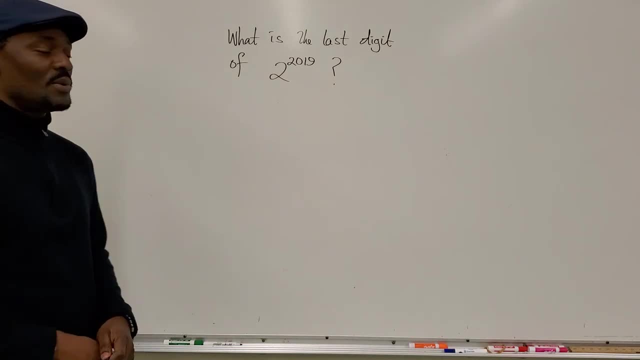 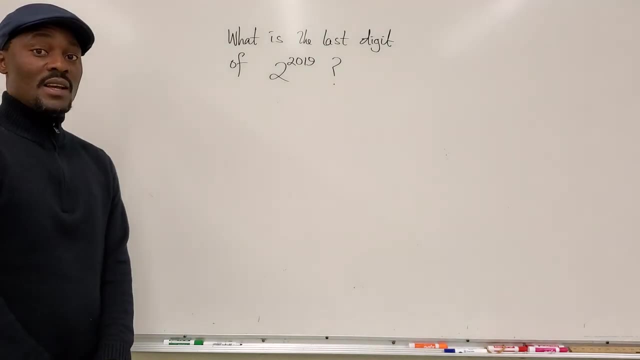 might be a tough question, but it is not an impossible question. It's very easy to solve if you have learned your rules of exponents. Okay, so I'm going to go ahead and show you the quick trick to solve this. And then there's. 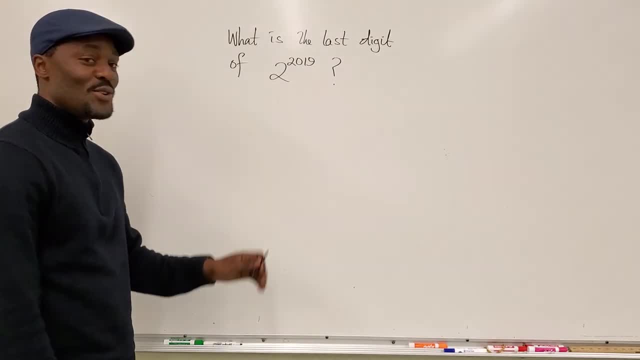 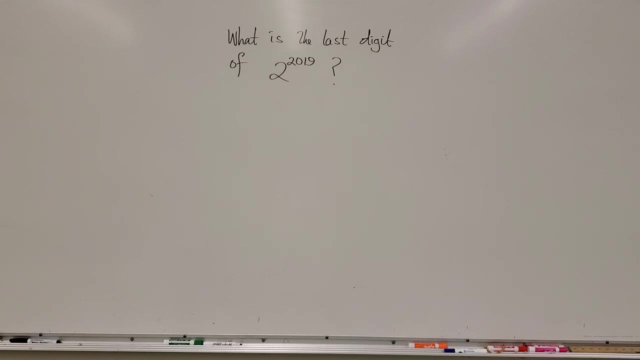 so many other questions, I'll give you one question also to try, after you've learned how to solve this. So let's go ahead and solve this. I just want to make sure this video is recording so I have not wasted all this precious time. Give me a second, We're good, Okay so? 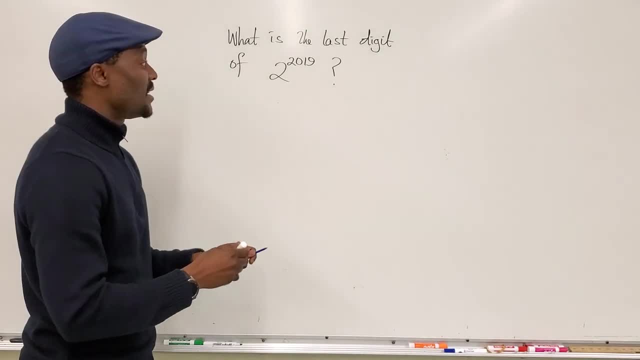 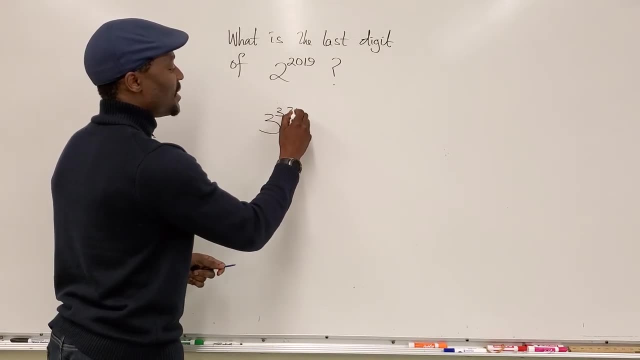 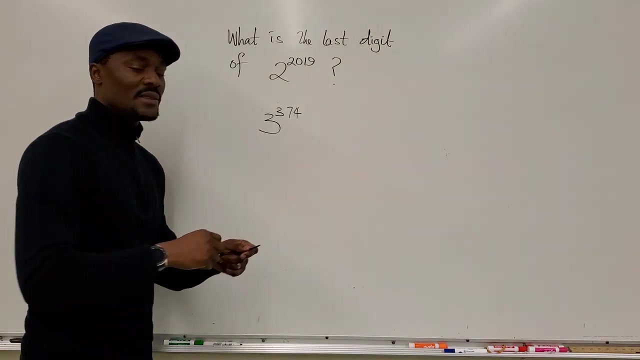 every time you get a question like this- I've seen other questions that look like this- You might get a question that says What is the last digit when 3 is raised to the 374th power Questions like this. you wonder: how are they? how am I supposed to know this? That is this method. 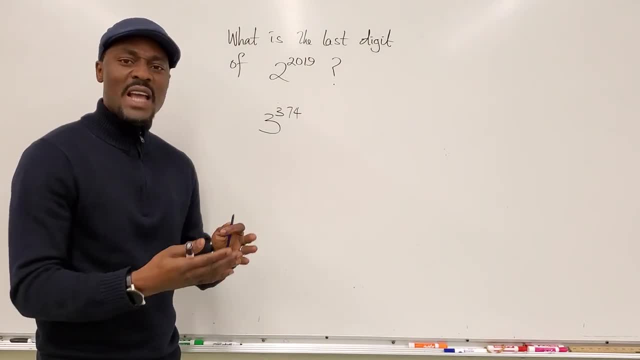 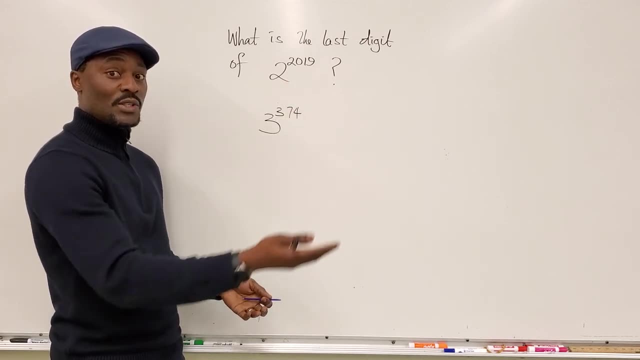 of solving math, which is called iteration. Okay, you just, you just need to list out. you start from what you know and you can predict what you don't know. So we're going to start from what we know and get to what we don't know. 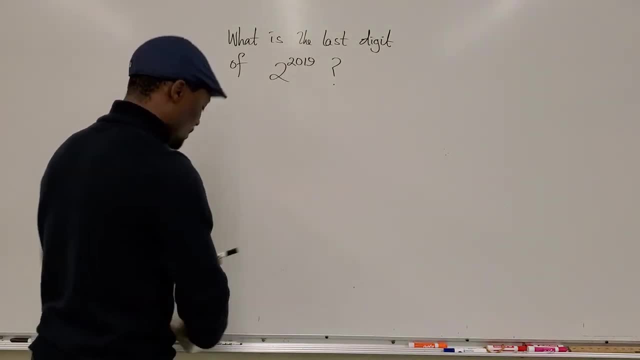 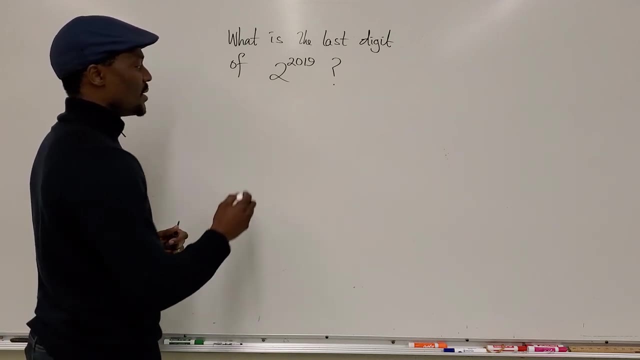 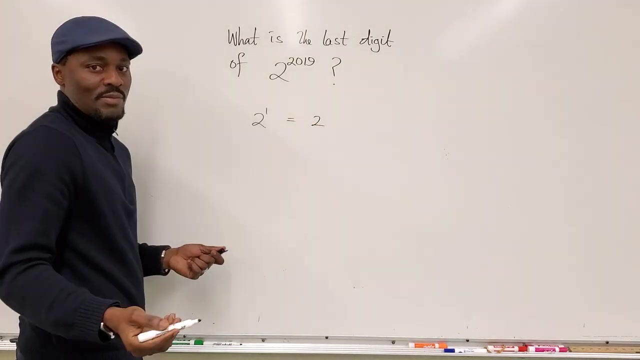 So let's see what we know based on this question, And then you can apply the principle to solving any other question that you come across. So the first one: we know that 2 to the first power is going to be 2.. That's 2 by itself. 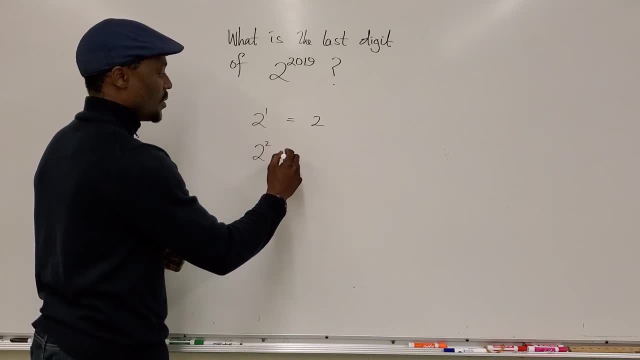 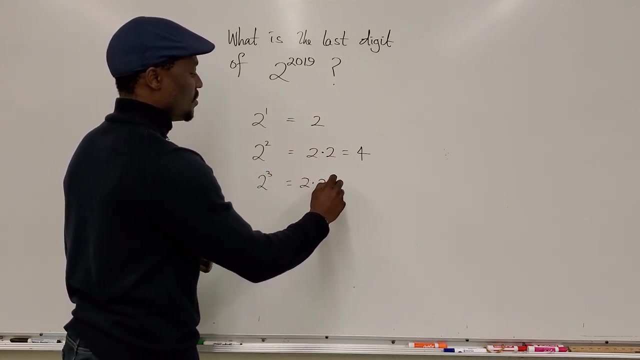 And then 2 to the second power will be the same thing as 2 times 2, which gives us 4.. And the last digit of your answer is 4.. Let's try 2 to the third power. It's going to give us 2 multiplied by 2, multiplied by 2.. 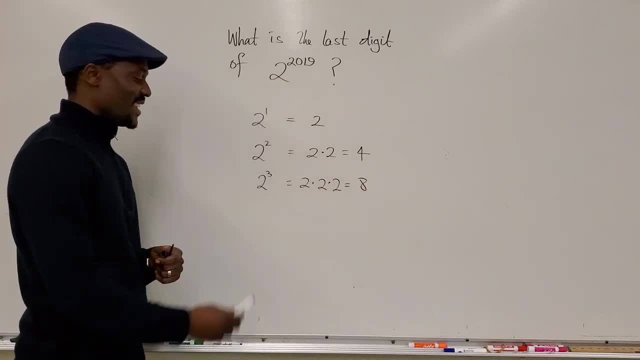 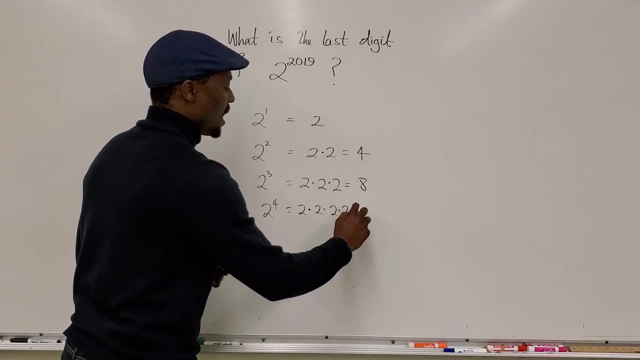 That gives us 8.. Now the last digit is 8.. Let's move on to 2, to the fourth power. That is 2 times 2 times 2 times 2.. And that gives us 16.. However, the last digit is just 6.. 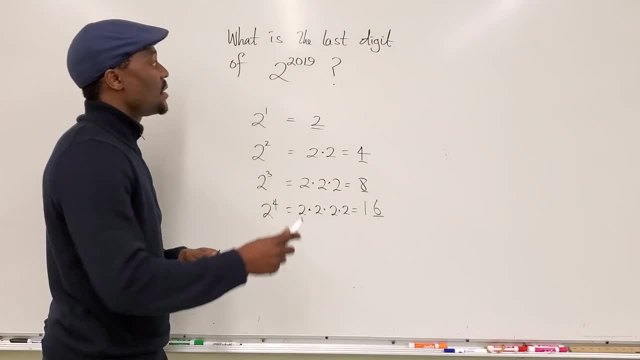 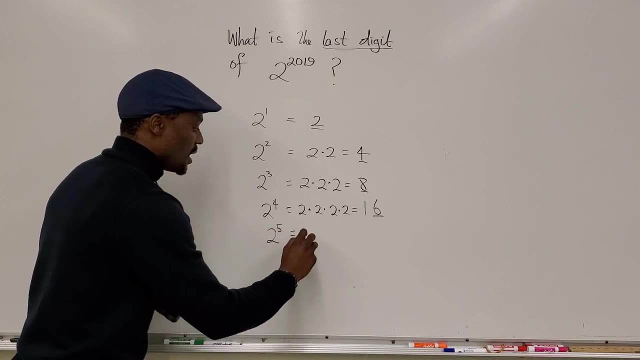 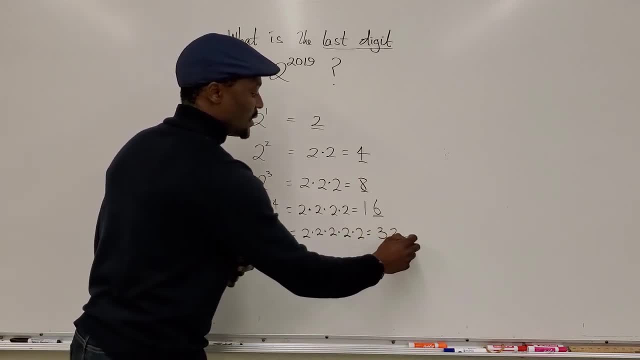 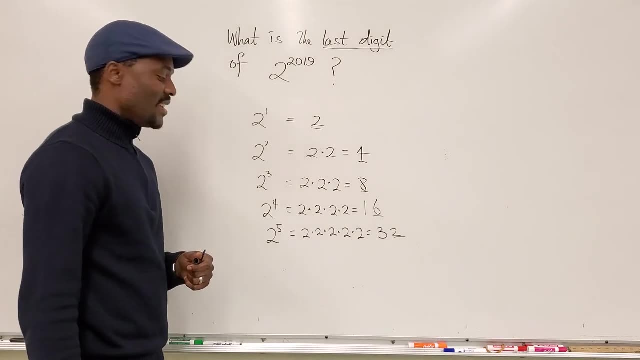 Your answer is 32.. The last digit is 2.. If you make an observation, it looks like we've gone back To this 2.. Well, let's see if we're right, Let's move on and do 2 to the sixth power. 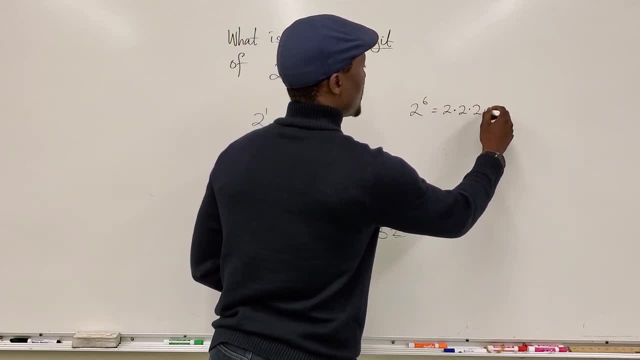 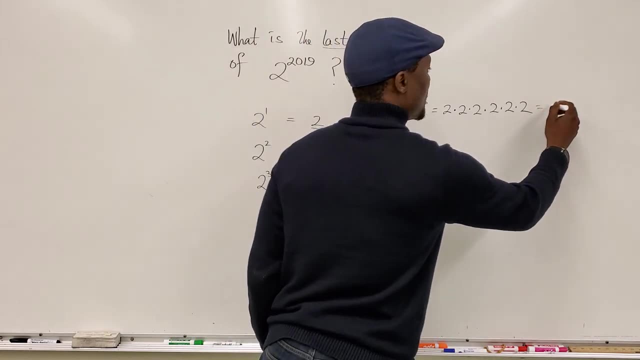 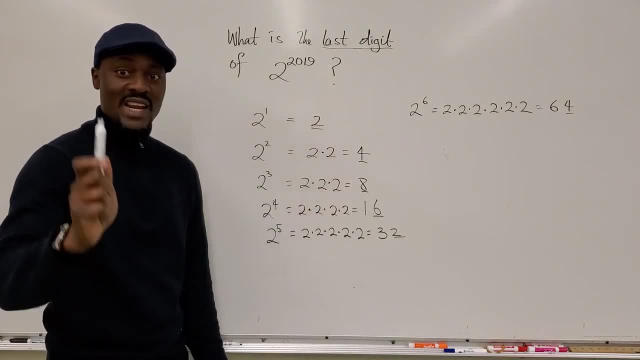 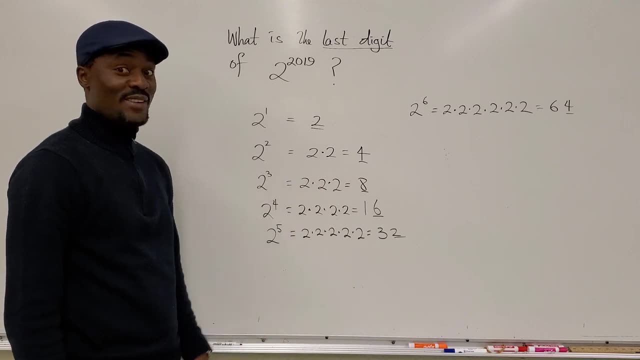 So we've gone to 2, 4.. We can predict that the next last digit It's going to be 8. And if that's the case, it looks like we're trying to find the rule. We have found the rule. 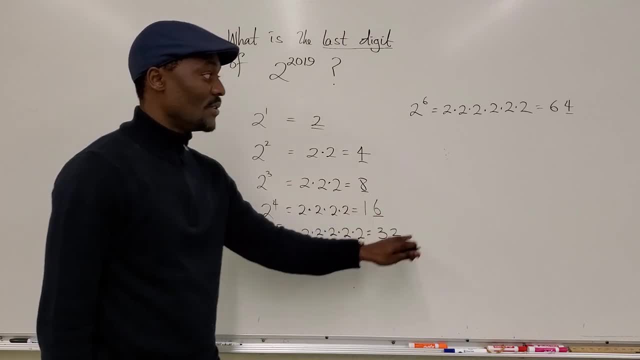 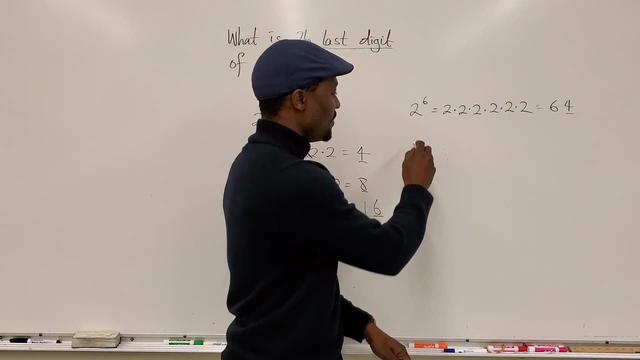 It's going to be 2, 4, 8, 6, 2, 4.. The next one should be 8.. Well, we can easily find that out. If you multiply 64 by 2, which gives you 2 to the seventh, your answer should be 128.. 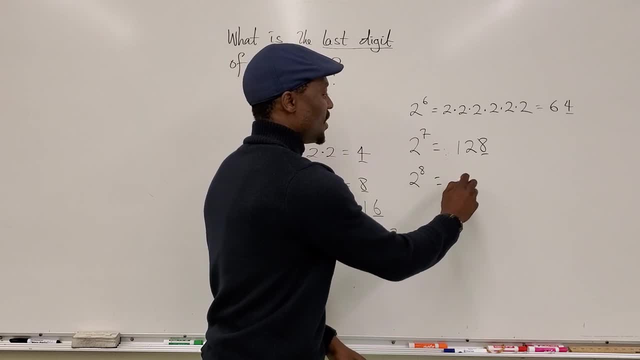 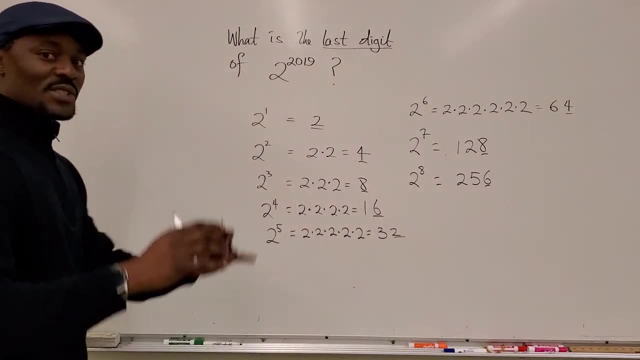 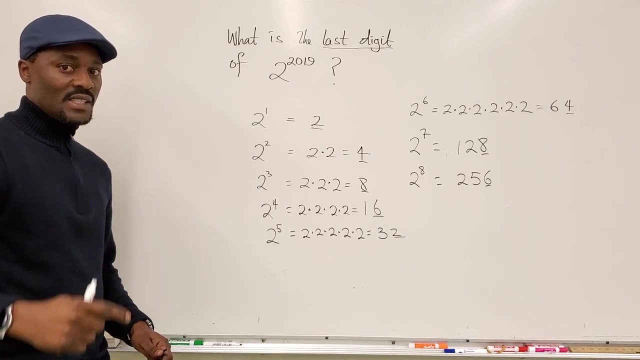 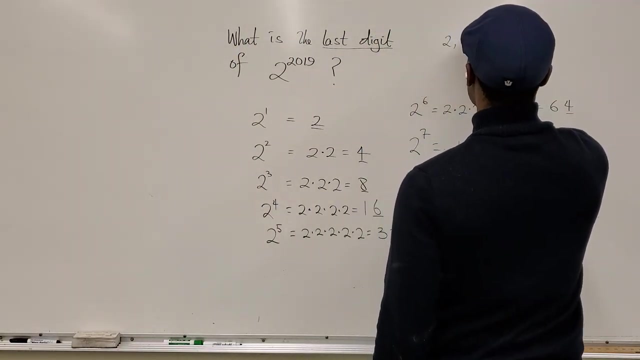 The last digit is 8.. If you go 2 to the eighth power, you get 256.. That's the answer. So you see that there is a cycle of four digits that keep repeating. OK, the four digits keep repeating and we have the cycle of 2, 4, 6, 2, 4, 8.. 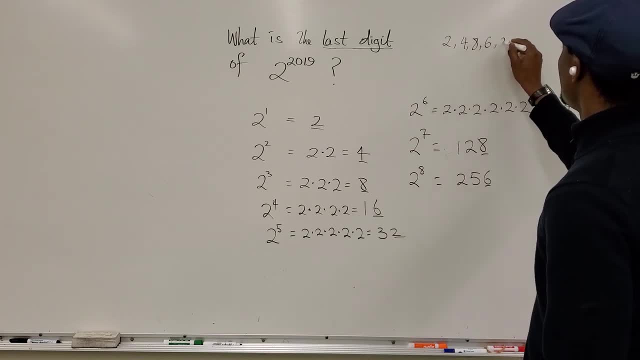 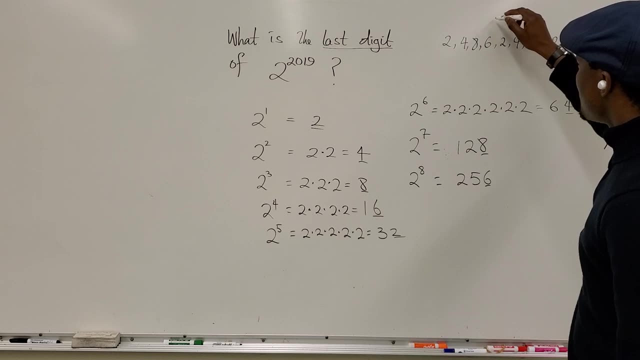 Excuse me, 2, 4,, 8,, 6,, 2, 4,, 8,, 6.. And the cycle repeats again too, like that. So there is a cycle of four digits repeating. Every cycle has four digits. 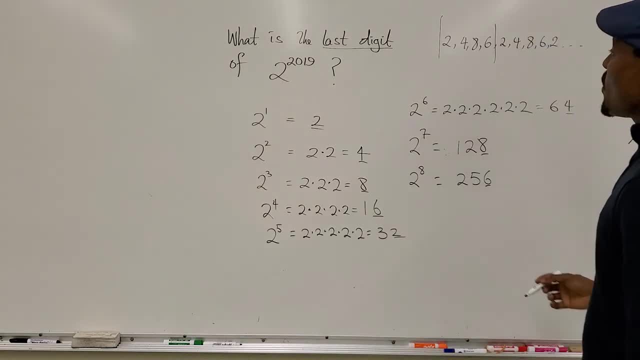 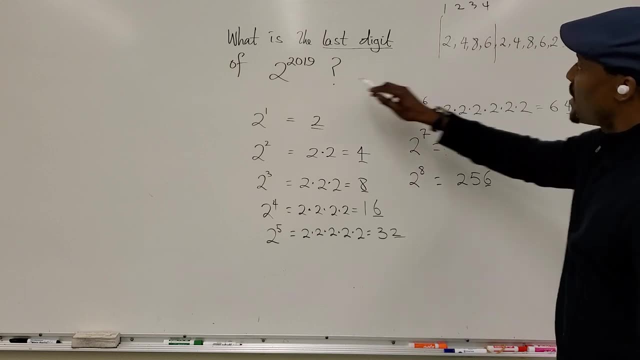 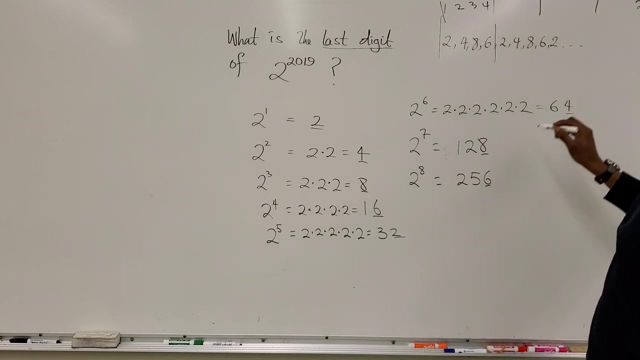 That's the secret. So, with that, all you have to do is say how many cycles of four You see. this is it. You start from 1, 2,, 3, 4.. By the time you get to 2019, you've done a cycle of 4 and 4 and 4.. 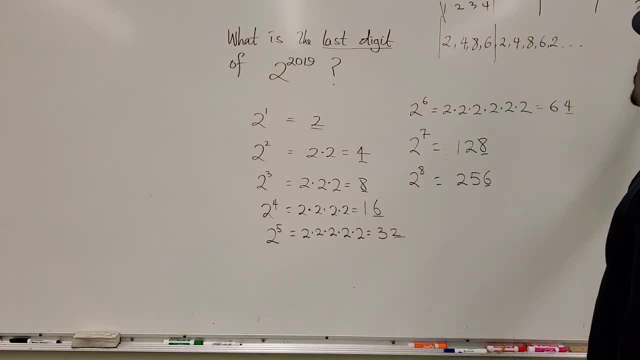 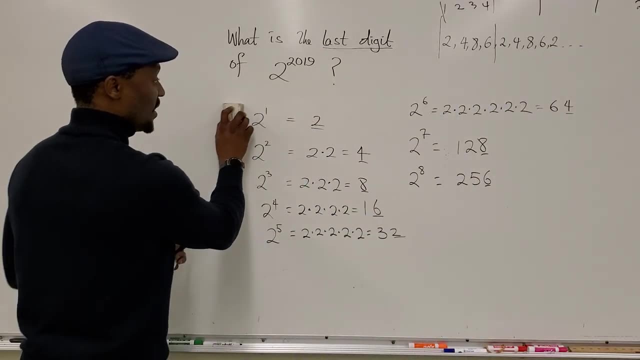 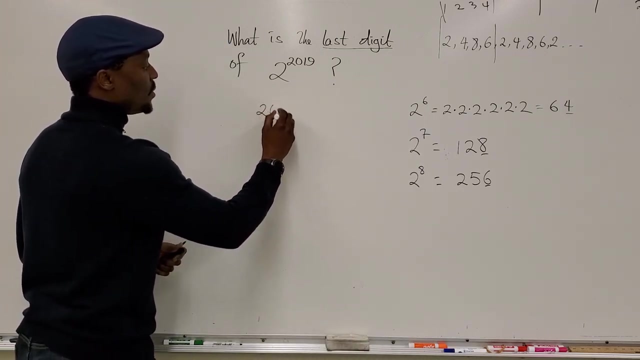 How many cycles of 4?? How many cycles of 4 will you get in 2019?? That's the beauty of the question. You just come over here. Get rid of this. Ooh, Now we've got. 2019 will have many cycles of 4.. 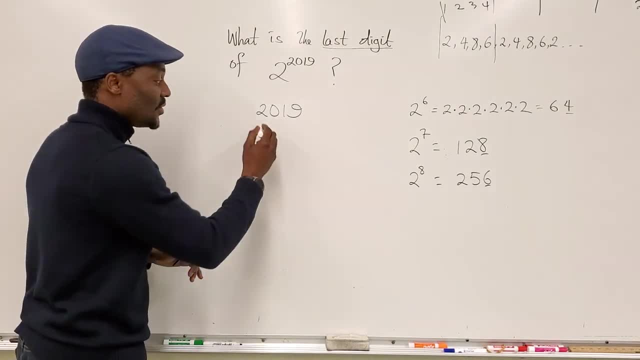 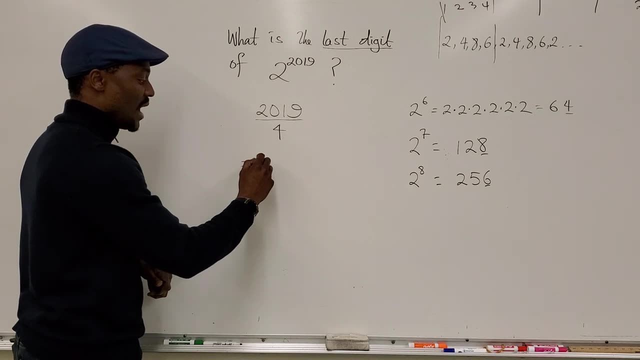 If you want to know how many cycles you're going to get, you just divide this by 4.. If you divide this by 4, how many cycles you're going to get? How many cycles you're going to get If you divide this by 4, your answer is going to be 5, 0, 8.. 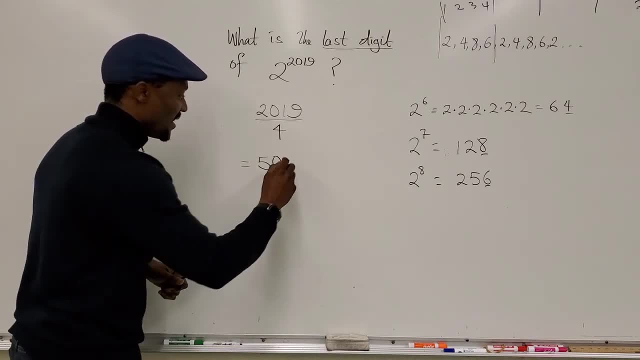 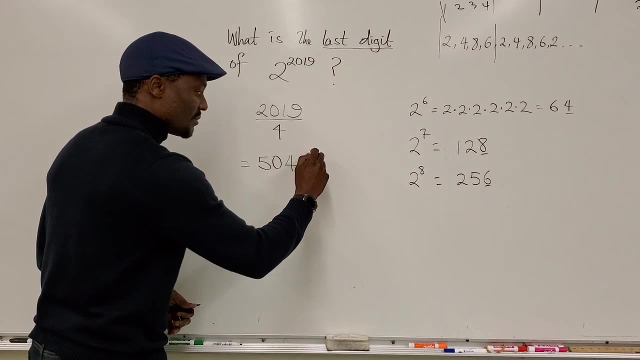 How many 4s are there in 2019?? Ah, It's going to be 4.. What's left? There's going to be 3 left. So there's a remainder of 3.. So there's a remainder of 3.. 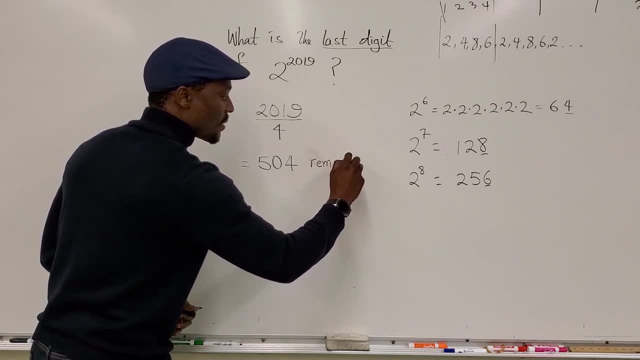 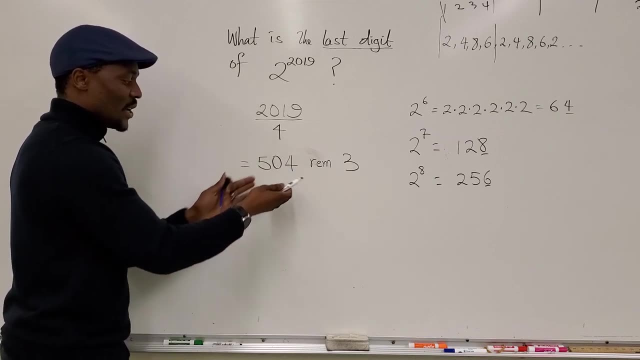 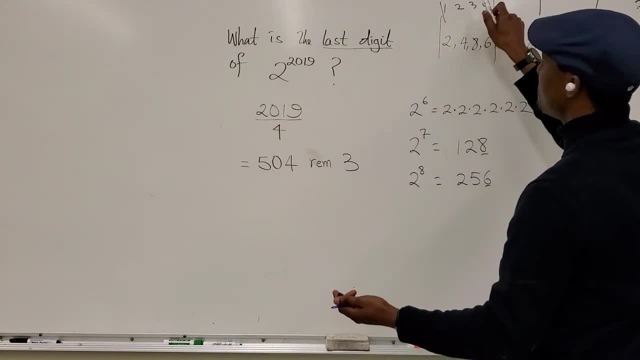 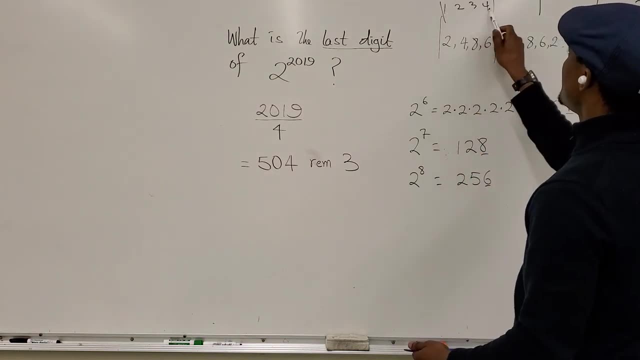 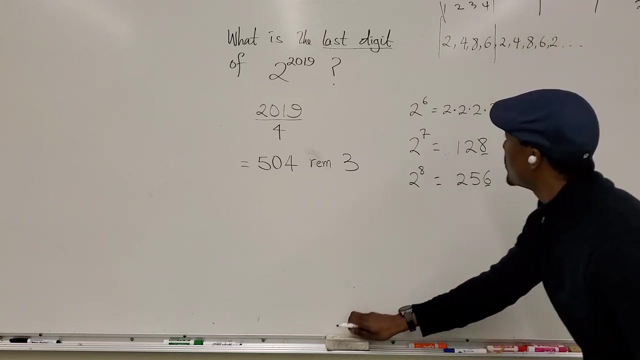 When you start another cycle- 1,, 2,, 3,, 4.. So you're going to do that 504 times. When you get to the very last time, when you get here, another cycle is going to start. So this is the 504th cycle. 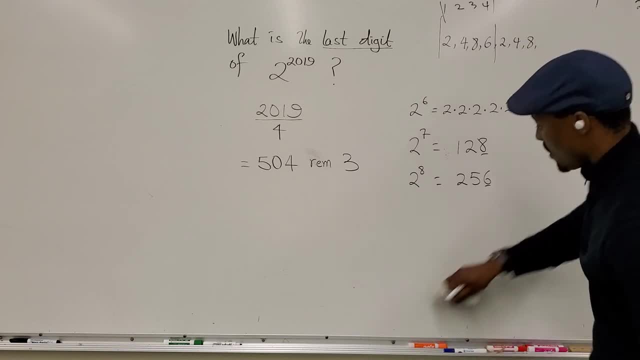 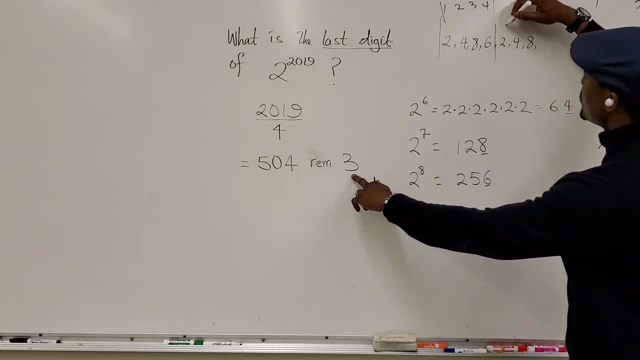 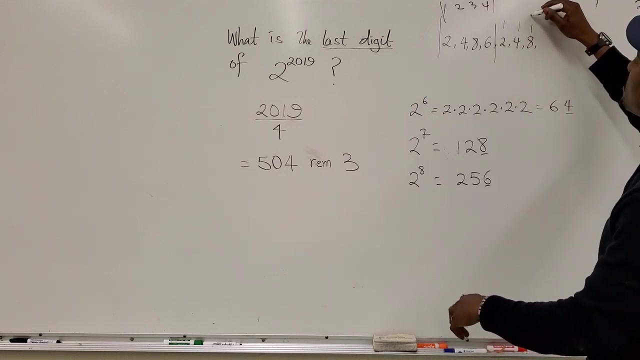 Let's assume this is the 504th cycle. So what does 204 mean? So this is the 504th cycle and then a new cycle starts, but it has three, So it would be one, two- this is the third in the next cycle, and this is where we're going to stop. 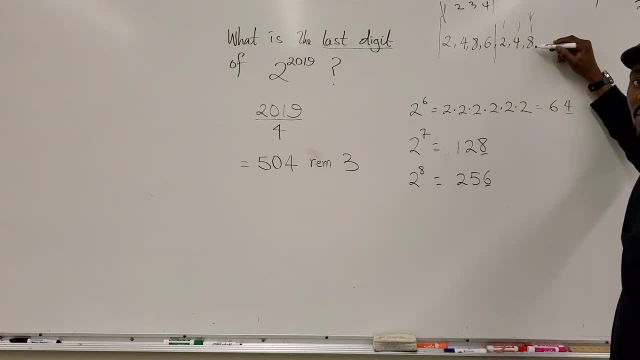 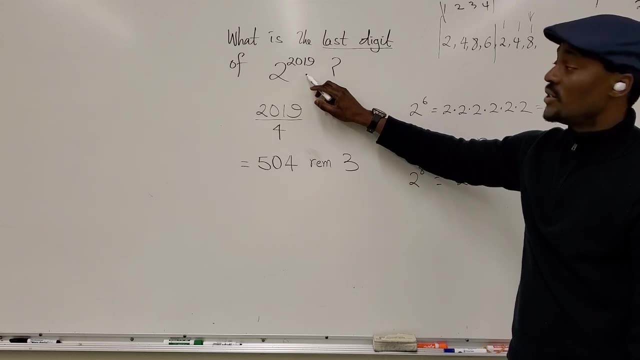 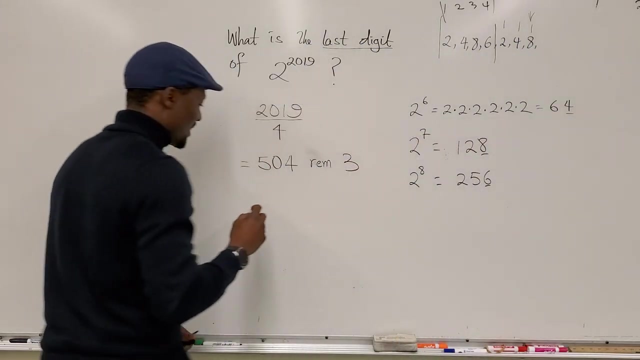 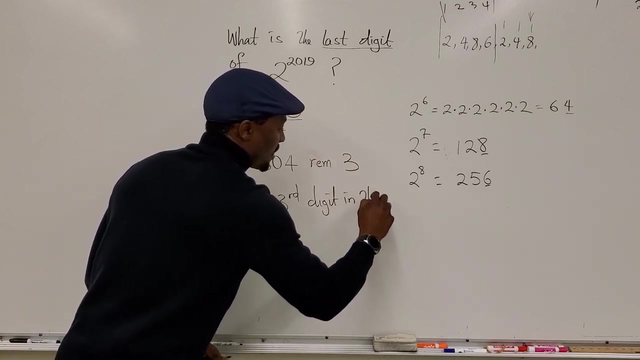 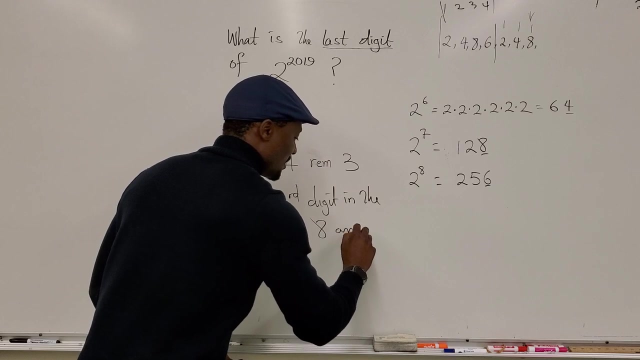 That tells us that the last digit in this cycle is eight Eight. The last digit of two race to the power of 2019 is eight. We found it, That's it. That's it. The third digit in the cycle is eight, and therefore, 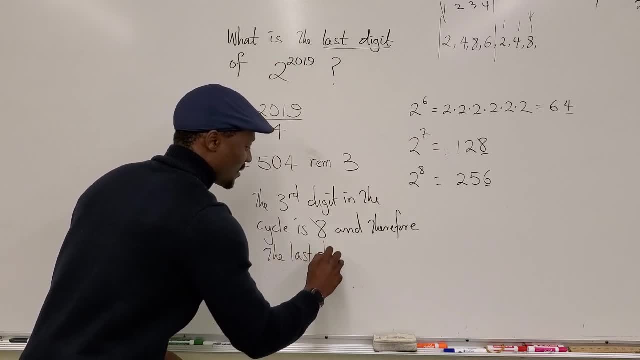 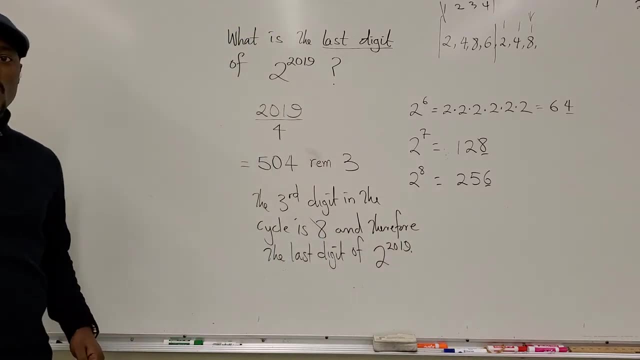 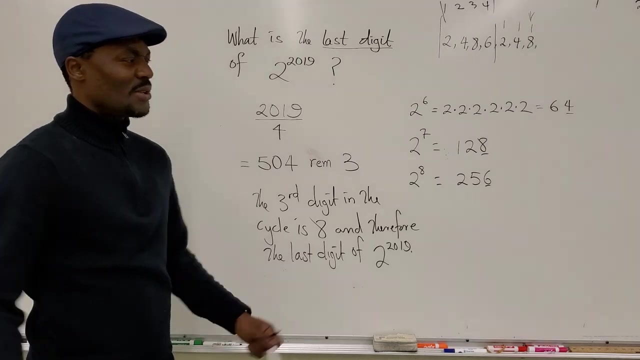 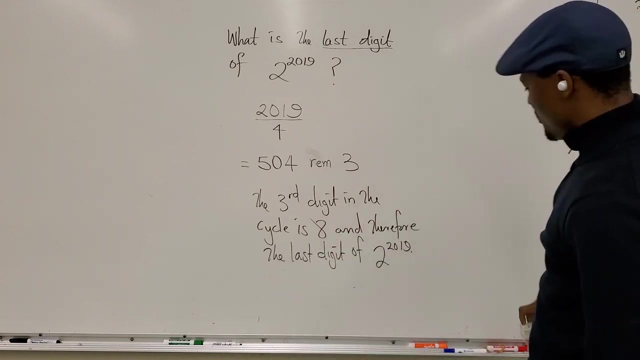 the last digit of two to 2019.. Whoops, We found the answer. Okay, Now let's test it on another number. Just a random number. I'm just going to pick a number and do something interesting. You can do it too. You know what? Take a pause, Try it. 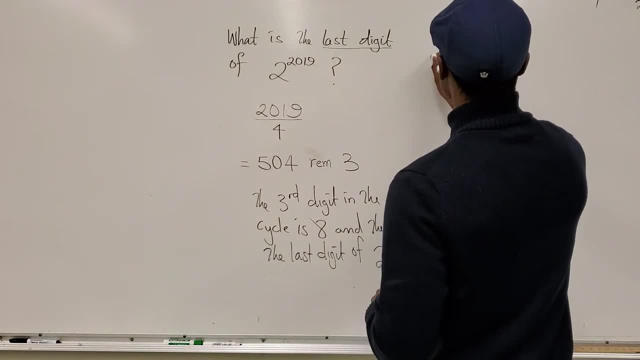 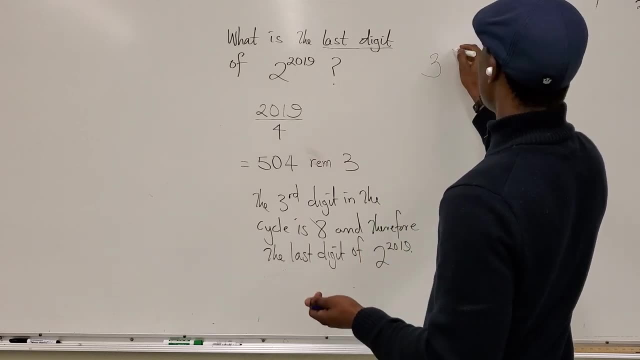 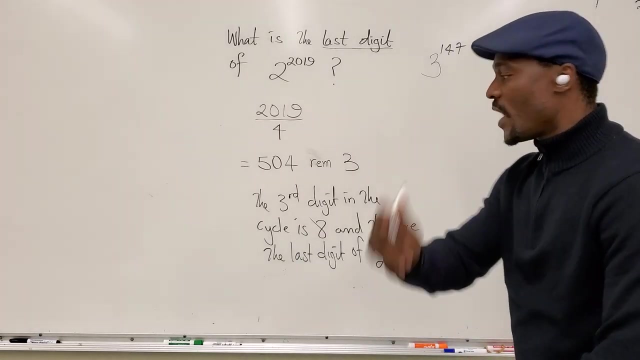 Pause this video And tell yourself what is the last digit of three to the power of, let's just say, 147.. See, that's easy: Three to the power of 147.. It's quick: All you have to do is create your cycle. 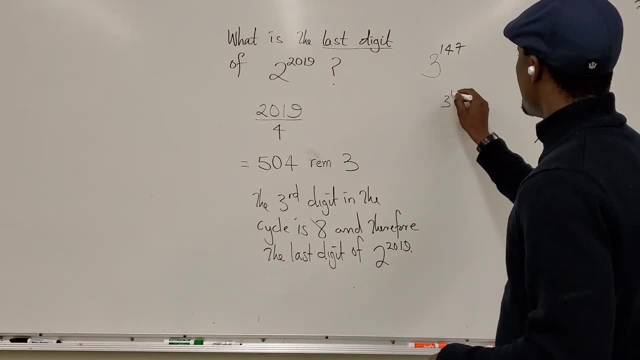 See how long the cycle is. So I'm going to go. three to the first equals three. three to the second equals nine. three to the third equals 27,. and three to the fourth equals nine. Three to the first equals nine. three to the third equals 27,. 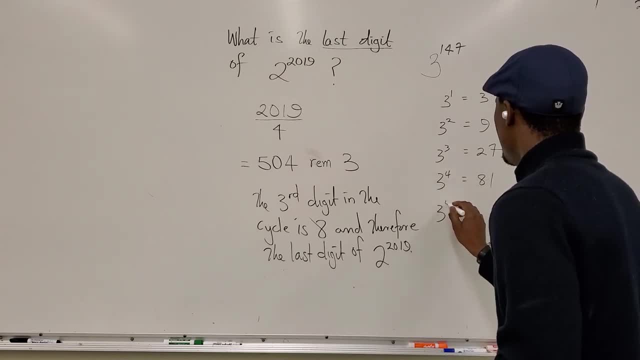 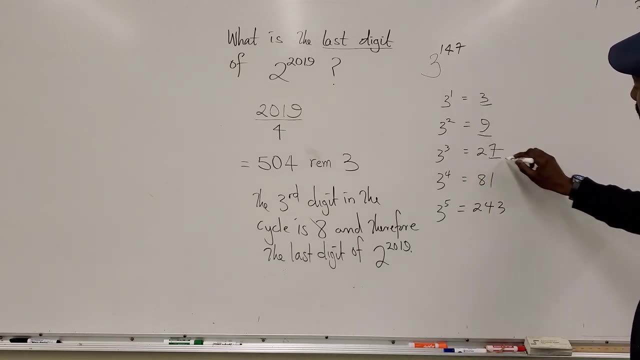 and three to the fourth equals 81, and three to the fifth equals 243.. Okay, So my digits have gone from three nine seven one. It goes back to three, So it's another cycle of four, You see. So the cycle is three nine seven one. 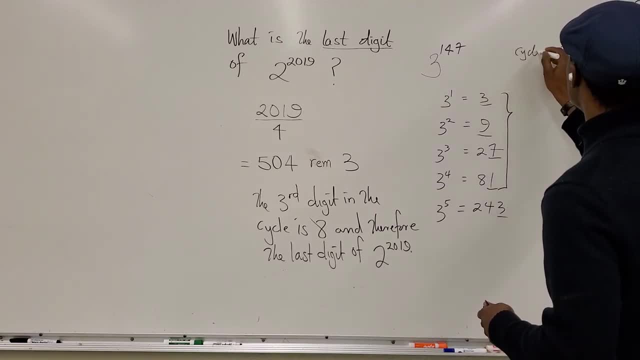 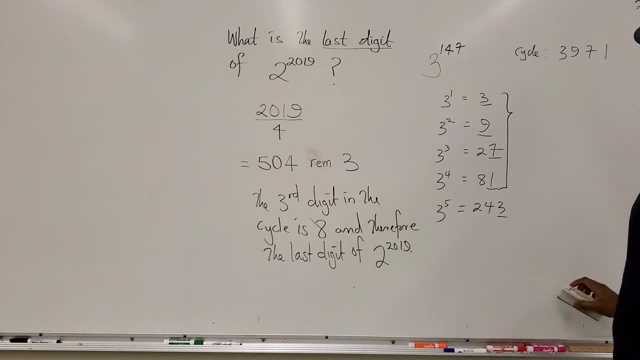 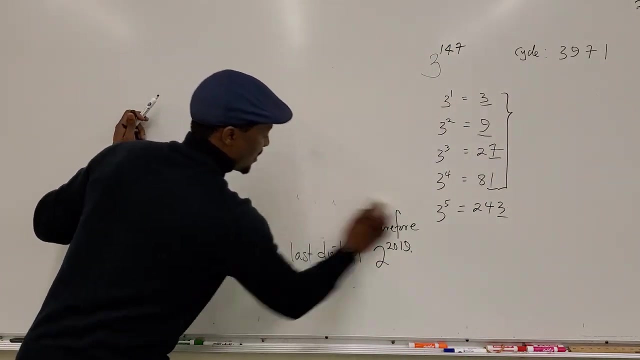 Okay, That's my cycle, So the next thing to do is basically go back to the original question. I'm just going to erase this. Okay, We're done. We're done here. Okay, So three, one, four. 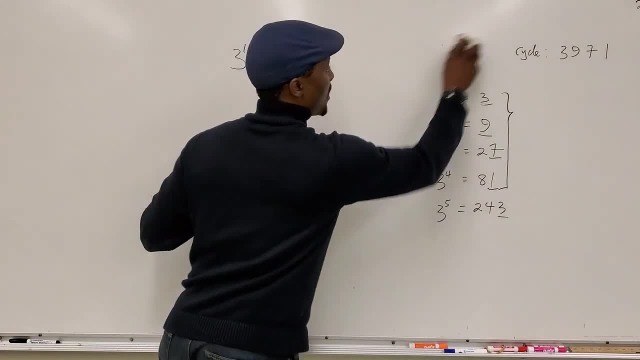 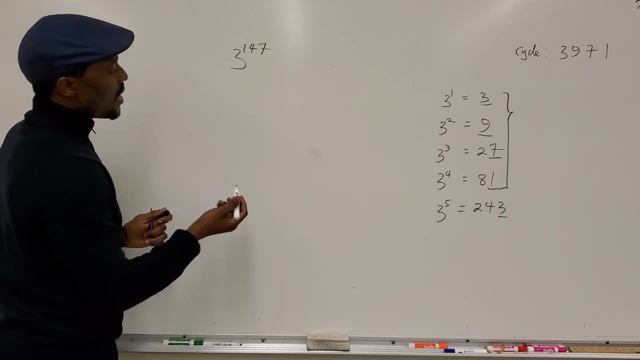 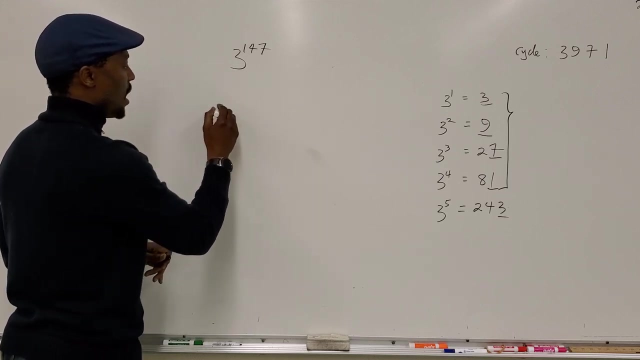 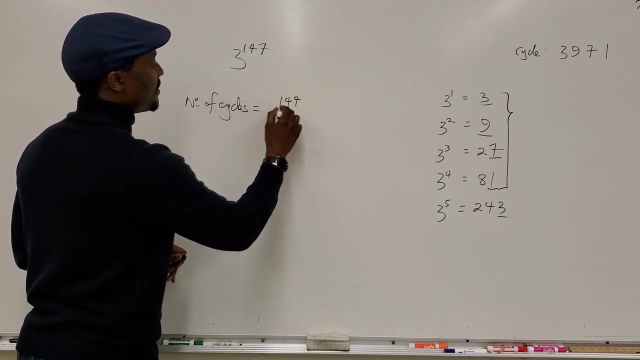 three to the power of 147. to well, give us, excuse me, will give us a cycle. The cycle is four. So how many fours will we get in 147?? The number of cycles will be: number of cycles will be 147 divided by four. 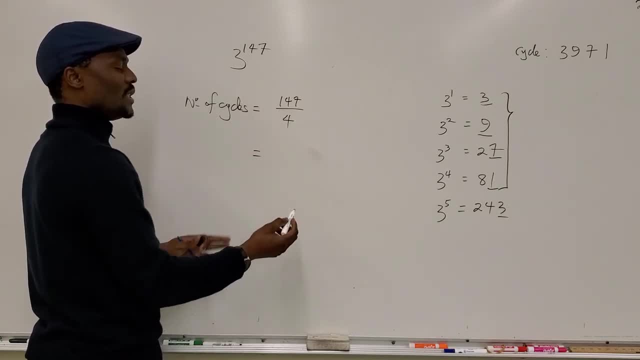 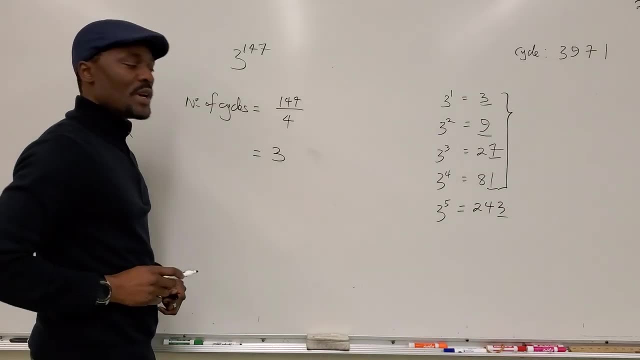 And that gives us four in 14, that's a three, leaving me with the two and the 27.. Four in 27 is 24.. Ooh, that's another one. Okay, It leaves it with a remainder of three. 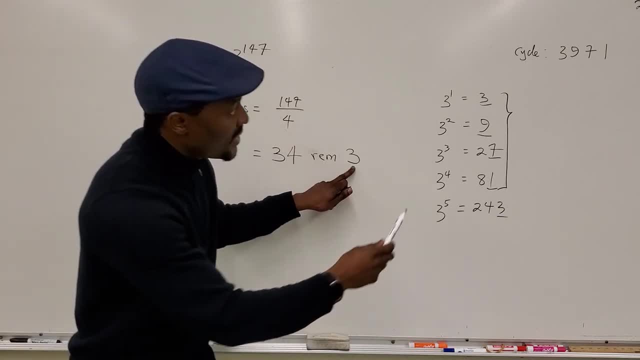 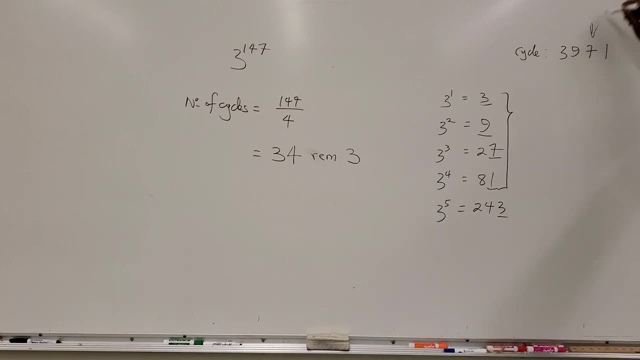 If there's a remainder of three, the last digit has to be the third one. Okay, So that's a three, The third digit in that cycle, and that number is seven. This is my answer. This is my answer. This is my answer. 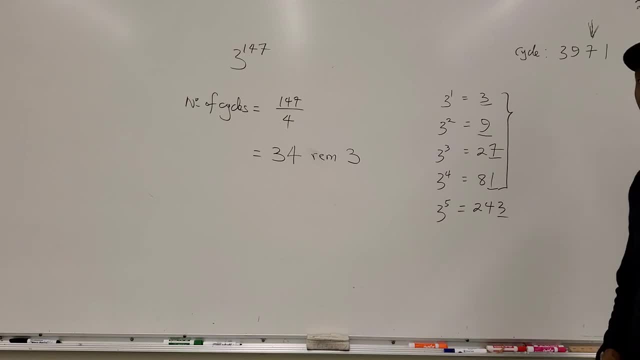 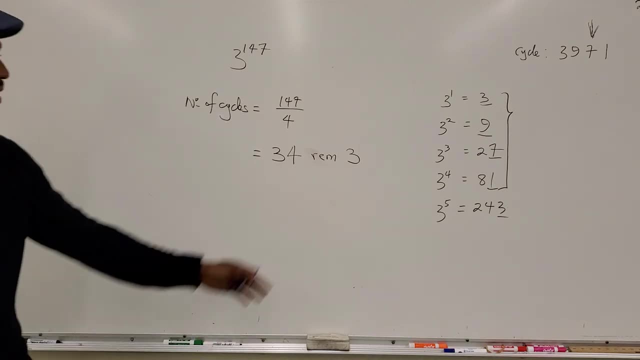 Okay, I hope you learned something today. There are so many other tricks, See, listen, you don't have to be a super math genius to solve all of these. You can see it's very easy for you If you've been through eighth grade. 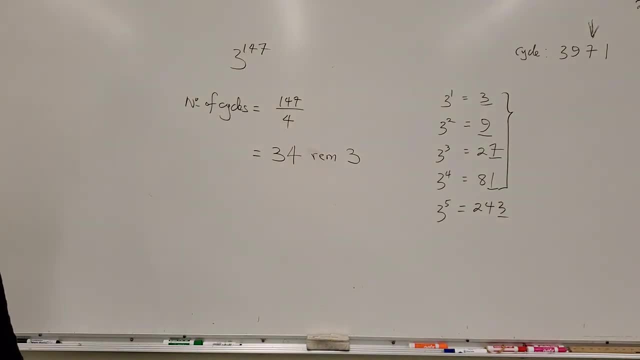 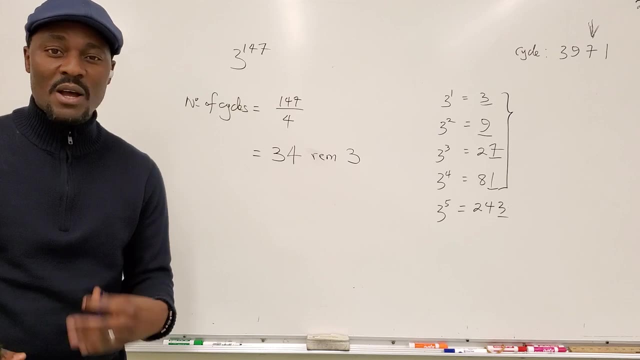 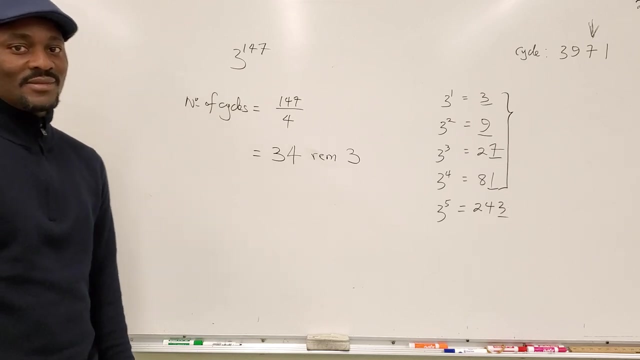 this is not a tough question. This is an easy question. Okay, Don't underestimate yourself And do everything you can every day to learn something new, Because he who has stopped learning has stopped living. Don't stop learning. So I'll see you in my next video. 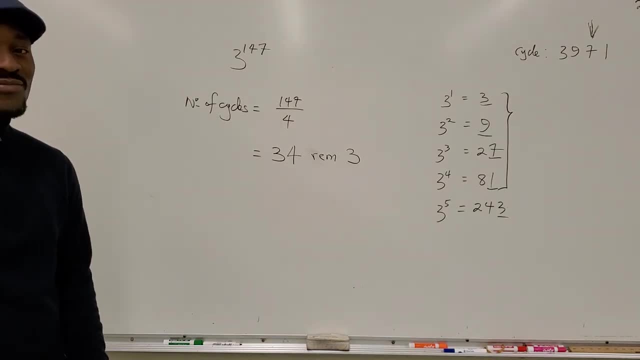 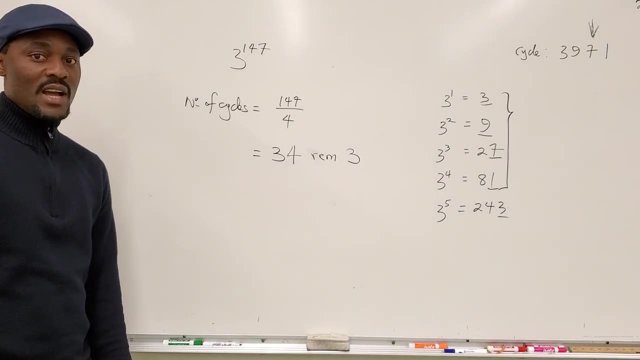 And in my next video I will be showing you another wonderful trick with the laws of exponents. Until then, have a great time. Once again, my name is Newton or KYA. Have a good time, Bye.